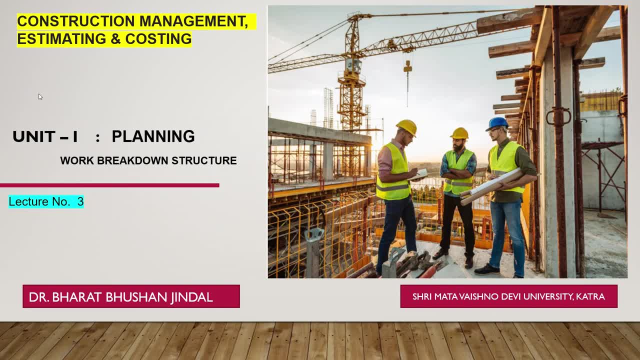 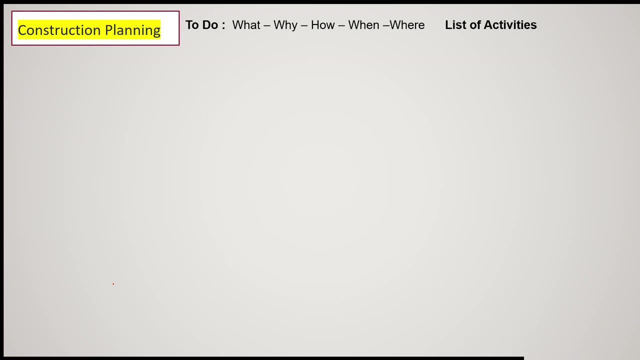 of all we have to understand what are the basic requirements of projects. That means what are the various construction activity which we have to go through. So first of all, today we will be understanding work brain structure. so in construction planning very important is: first of all we have 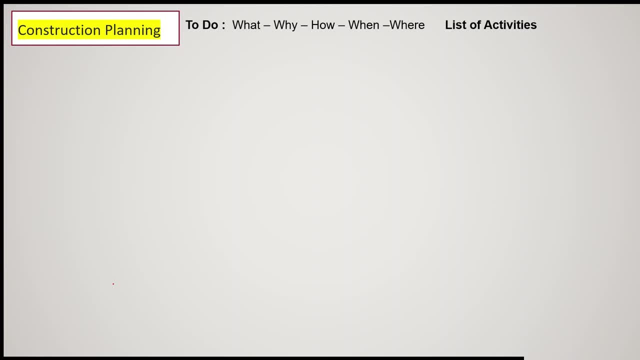 to list out that. what are the various activities which we have to do during the construction project, why those activities we have to do, then, how those activities can be accomplished, when that mean timing. we have to check when we have to execute those activities and where we have to do all these process. 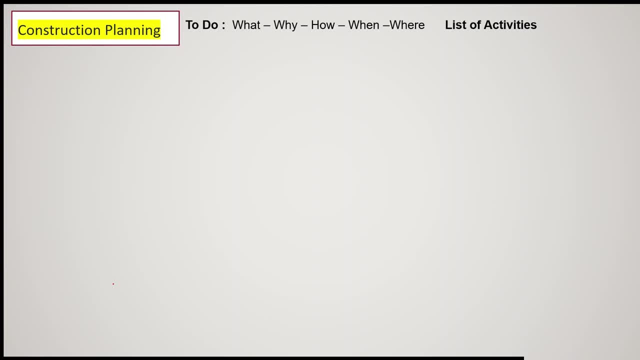 so, in brief, we have to list out to the various activities, or list of activities we have to prepare. then we have to go through the detail, so which activity we can start with and which activity will be followed, and what are the various activities which we can run in parallel to each other. 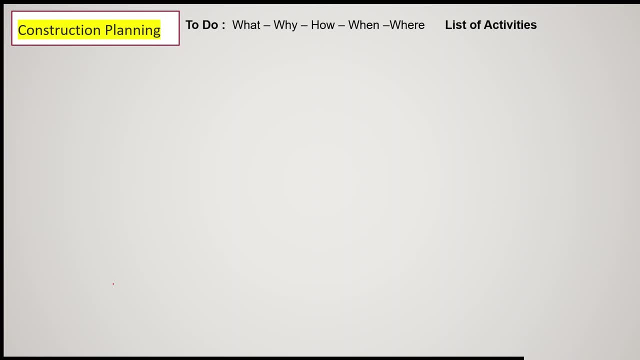 So whether one activity depends upon other activity or not, whether one activity depends or can only start with the completion of first activity, or whether it can start midway or in parallel. So let us understand work breakdown structure. So whenever there is a big project, 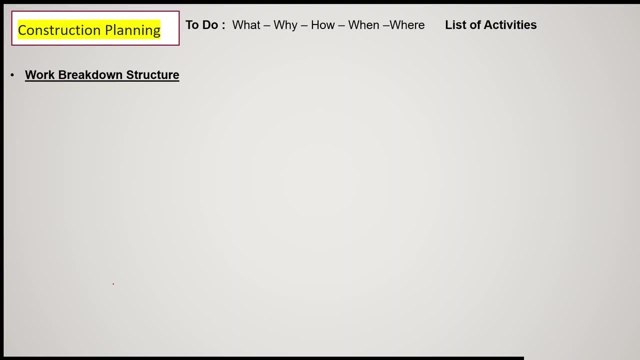 that big project will be first of all divided into various processes or you can say sub-projects. So for efficient planning, project is divided into various functional elements and their interrelationship are determined. So first of all, in whole, we have to get through the project and we have to divide. 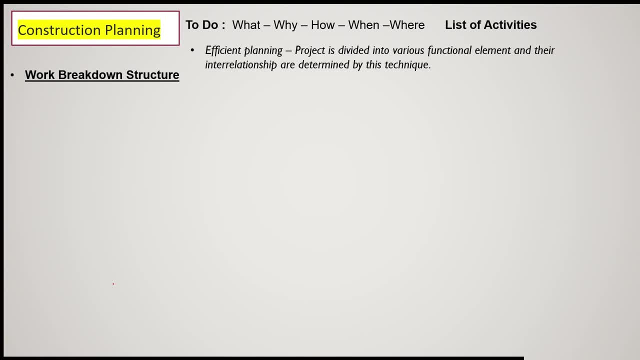 it into various functional elements. Functional elements, you can say, just like one element may be concreting, there may be surveying, there may be exploration, like this. So each system is broken into subsystems And each sub-system again into some components And so on. we will be breaking down the system. 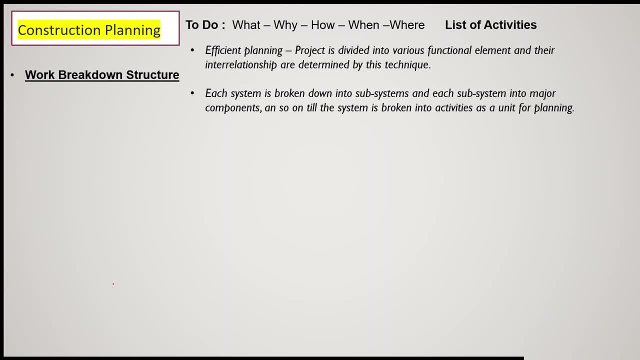 into subsystem and components, till the system is broken into activities as a unit for planning which we can plan, Suppose you have to do the excavation work, So excavation is let one system which you have to follow. and for that excavation, what are the various activities on? 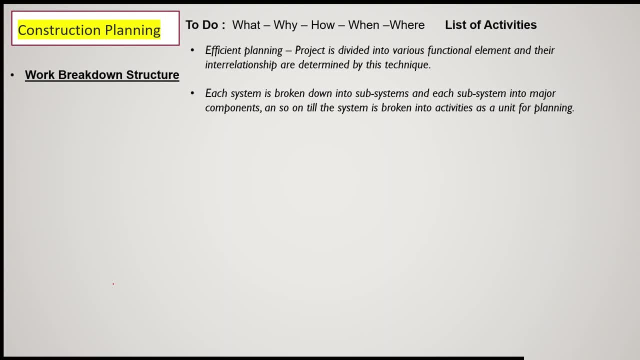 which excavation depends, and to complete the excavation, what are the various activities we have to perform? so let us take very simple example of a construction of a compound wall. so let us there. there is a project and we have to construct a compound wall. so here we have. 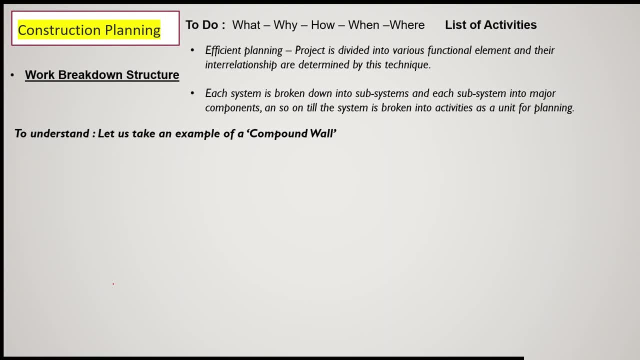 we need to understand that, how to proceed and what will be the completion point of the construction of the compound wall, so that compound wall will be divided into various activities. so first one, there is a compound wall now here to execute the construction of compound work. what we have to do? we may have to do the excavation. there may be some concreting, blasting. 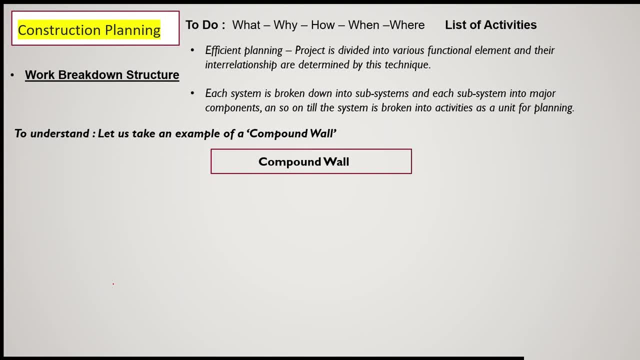 etc. so all activities we have to list out. so here, very first activity will be excavation for a compound work. first of all we have to excavate the soil to construct the foundation of the compound wall. so excavation will be the very first activity. then second activity: after excavation we have to put the lean concrete in the foundation. 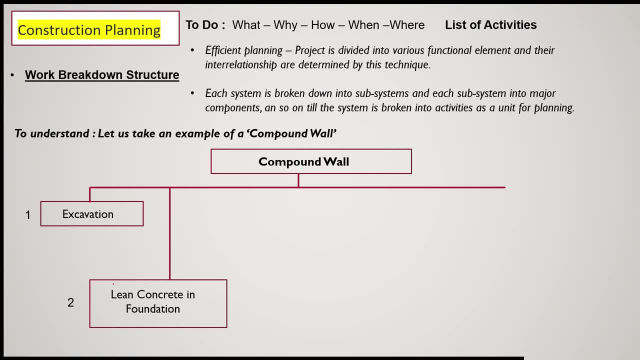 so now it is very much clear here that lean concrete will be the second activity and first activity will be the excavation. so leaning lean concrete- that means pouring of lean concrete in the foundation- cannot be the first activity. that means first of all you have to excavate, then you can proceed to the second activity. third one is masonry in the foundation. 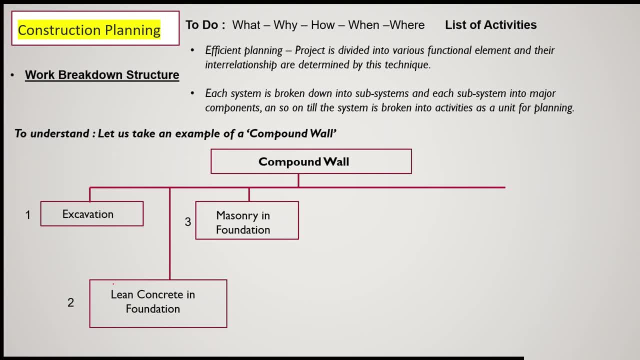 now you can clear understand from these activities in the foundation. now can clear understand from these three steps. step number three, or activity, can only start when activity two is completed and activity two can be only started when activity one is completed. so there is interrelation between these three activities. fourth, one will be after putting the machinery in the foundation up to the 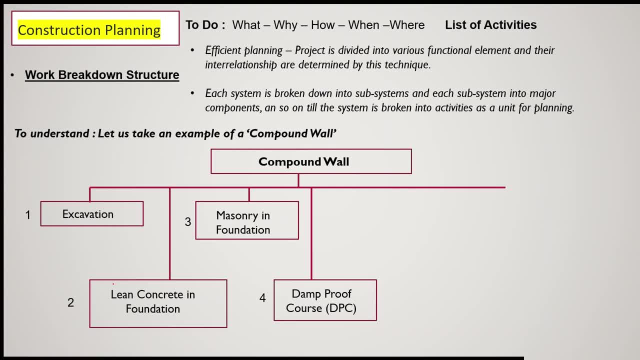 required level as per the drawings. then you have to go through the fourth activity, dpc. that is done. proof course. now it is very much clear. they are in order: one, two, three, four. no activity can be interchanged in this particular case. fifth activity will be after dpc. you have to construct the foundation wall. that is machinery in the super structure. 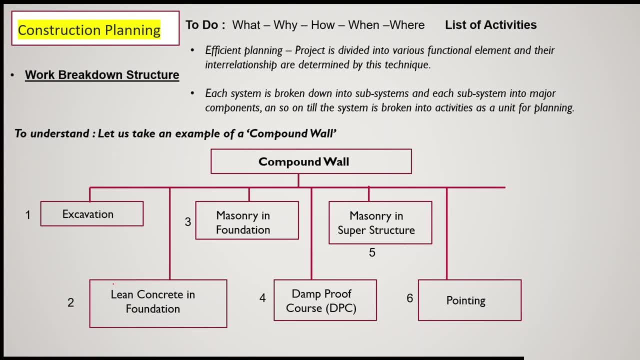 then sixth activity be pointing- now pointing cannot be done before the construction of the superstructure wall- and seventh will be copying. so here you can easily understand that there was one element. one element is compound wall and that element is divided into various activities. now excavation is one activity, as i have explained here. you have to broken down. 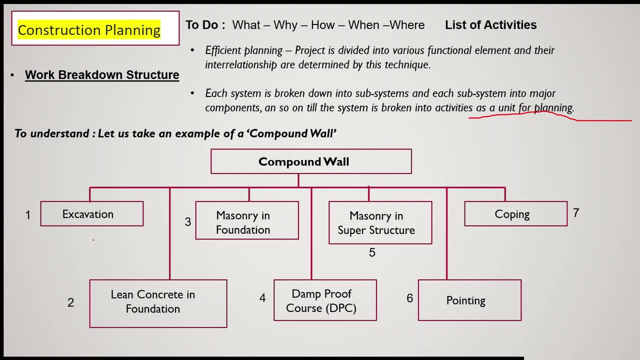 activities as a unit. now excavation is one unit, compound wall is one system or you can a subsystem, and that is divided into seven steps and each one excavation is one unit. that means if you say excavation, then everything is clear. so all these processes or activities, they have to run in the same order: one, two, three, four, five. 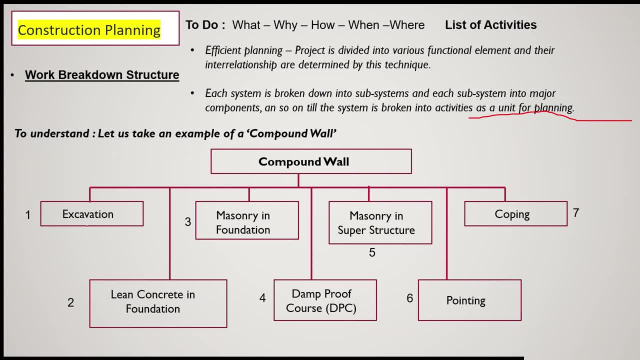 six and seven. so here, from this diagram, your flow chart, you are able to understand that which activity will be start activity and which activity will be the ending activity. so excavation is the start starting activity and copying will be the end activity. so in between all activities you have to organize in a systematic way. now suppose compound wall. 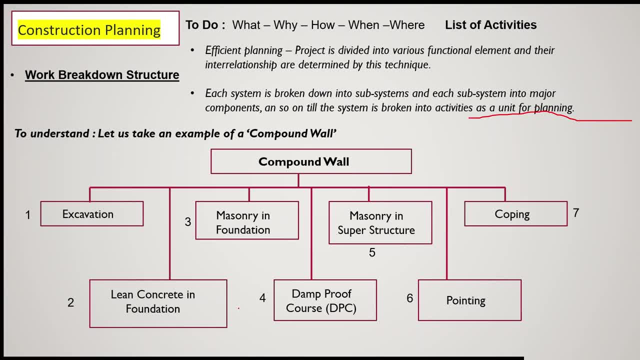 we have decided that it will take seven days. let us suppose seven day is the construction duration of the compound work. so if you, your excavation get delayed, then all the other activities may also have the possibility of delaying. so here you have to put all these activity in a particular time frame so that we can discuss, understand that, what is the duration which? 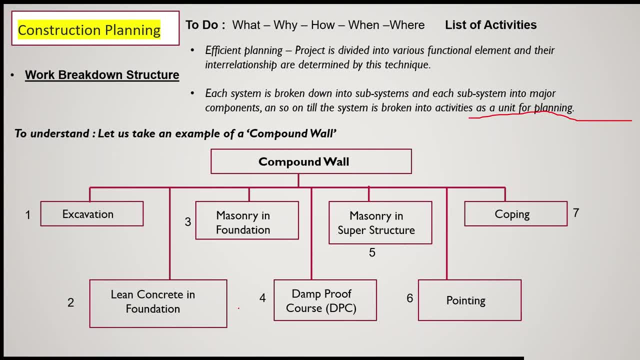 we have planned for the compound wall and whether that compound wall is affected by other activities. now, if you are constructing a compound wall and simultaneously you are putting the foundation within the campus, that mean then compound wall as well as the foundation activity of the any building which you are going to be constructed within the compound. 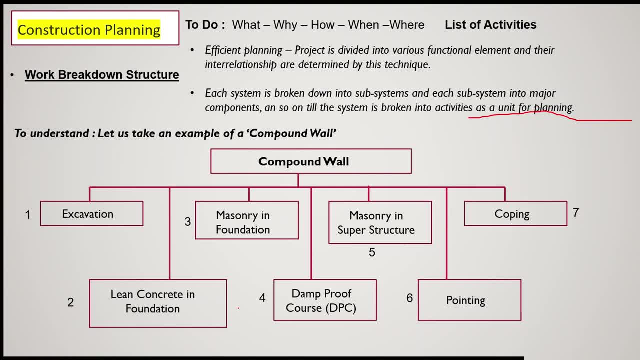 compound wall. they can run parallel, but compound wall cannot be started with the second number of activity, that is, lean concrete in the foundation. so all activity we have to understand. if we are able to different activities, we can divide thus whole project into systematic way in various activities. and then you. 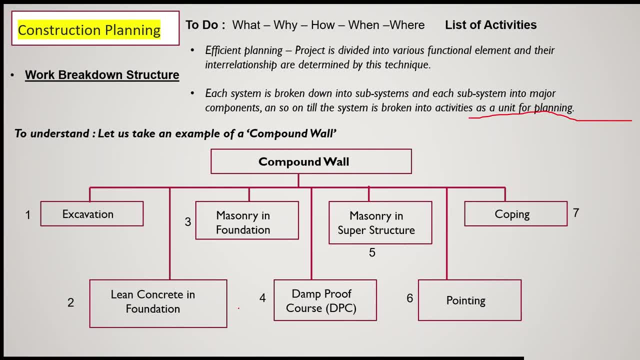 can just put a flow chart or a timetable you can decide, so that when and which activity we have to start and how much time it will take to complete that activity. so basically this comes under the plan. this is basically planning. now here you have planned the construction of the compound wall. similarly, in broader sense, you will plan 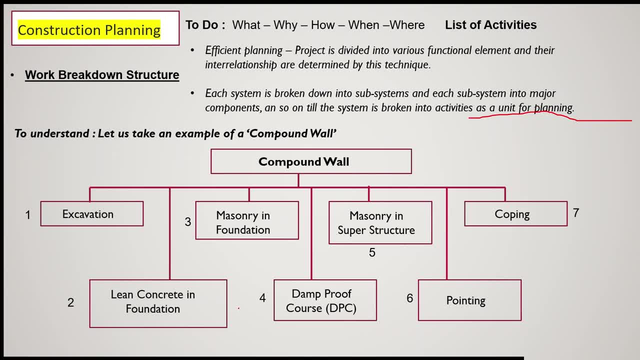 the execution of a project or project duration you will decide. so all activity you have to divide accordingly and you have to be very clear in planning which activity we can run parallel to each other and which activity you can start only at the completion of earlier activity. so this process is known as work breakdown structure. 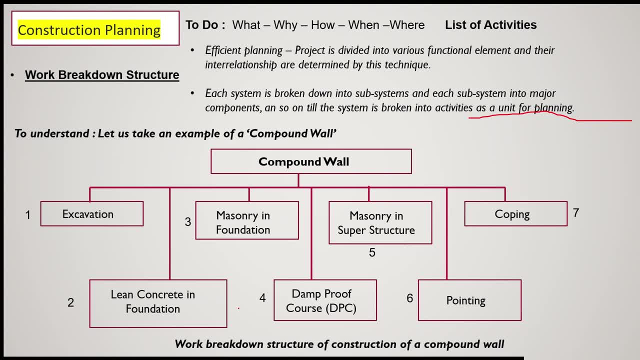 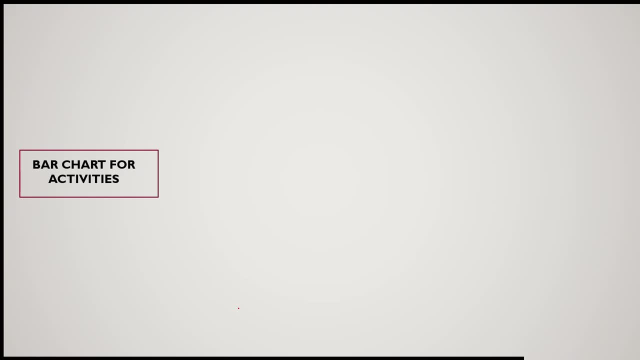 so we have to understand how to break down the complete work or major activity into smaller activities and so on. now how to arrange and how to represent duration as well as activity in a systematic manner, so that process is known as bar chart. this is the one methodology. 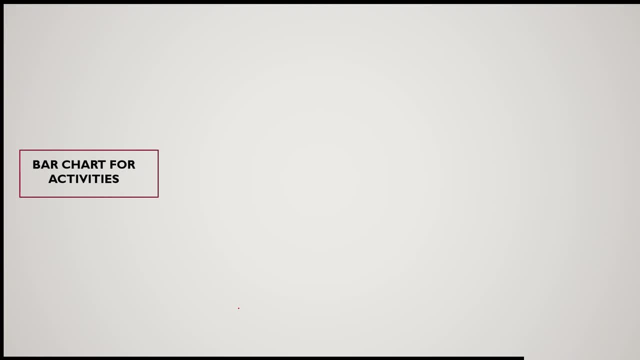 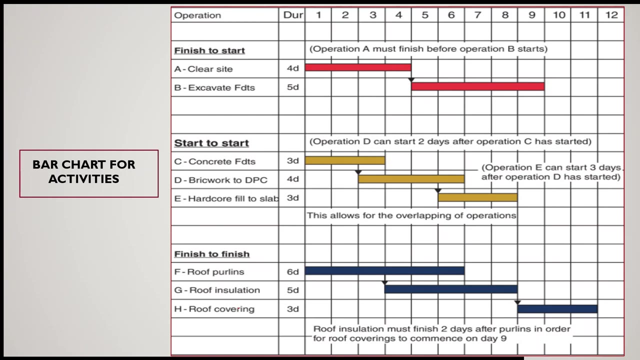 by constructing a war chart. and for your understanding, just for example purpose, i have taken one bar chart directly from internet which we can discuss now here. you can construct this bar chart even in excel or in any software. so what we have done, we have, first of all, 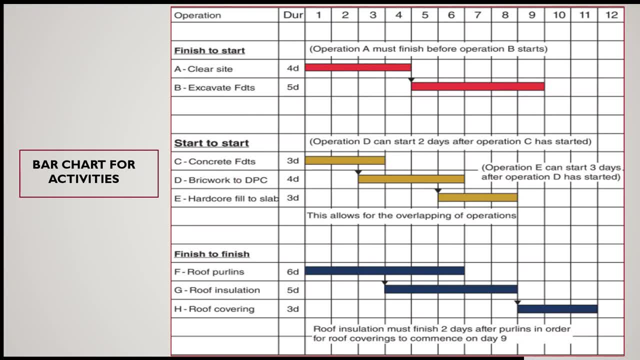 listed out the various operations or various activities, then duration, and then duration in a chart, one, two, three. like this: now, here, very first, is when you have to from finish to start. first of all, a activity, it will be the clearance of the site. first of all, you have to clear the site and let you have decided that it will take four days, so four. 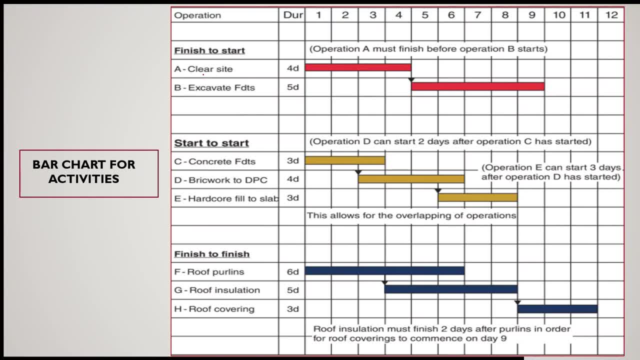 days we have given or assigned to clearance of the site. so that means you can start this activity from very start, that is, from zero day, that is, one day two, day three, day four. so you have put a bar here which is indicating that this will be the starting time of this activity and this will be 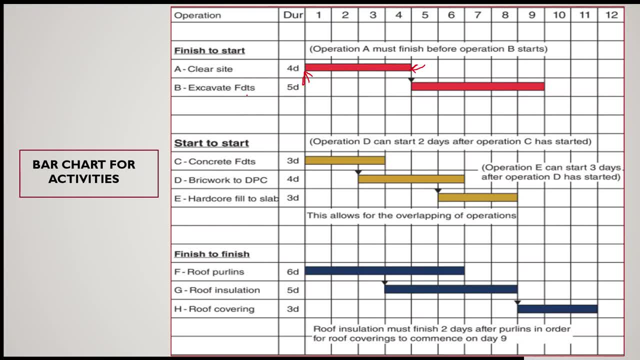 the completion time of this activity. then, after clearance, activity b is excavate the foundation. so if you have decided that we will be completing this excavation of foundation in five days, then this five days activity can only start after fourth day. you can't start it from here, so it